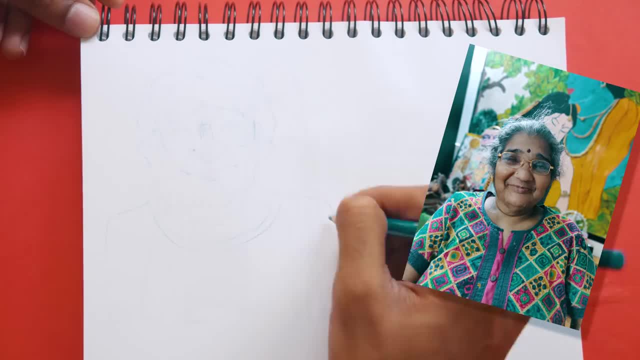 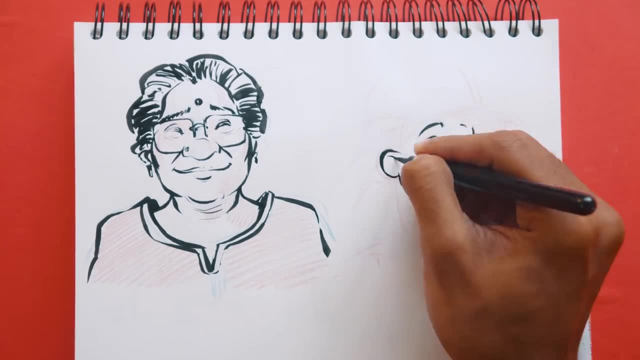 animes and all those other things are just personal interpretation of life itself. So instead of learning from those things, you can go to the very source and come up with something new on your own. And if you can't draw from life on a consistent basis, just draw from photographs. 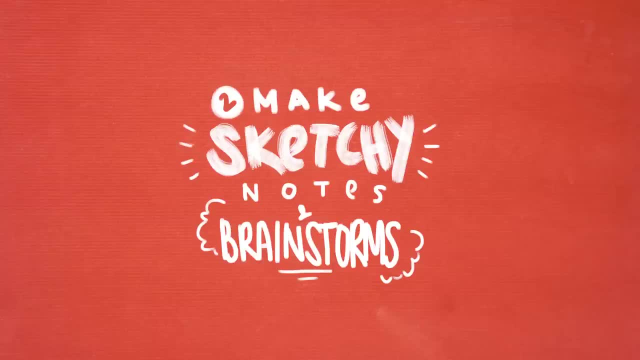 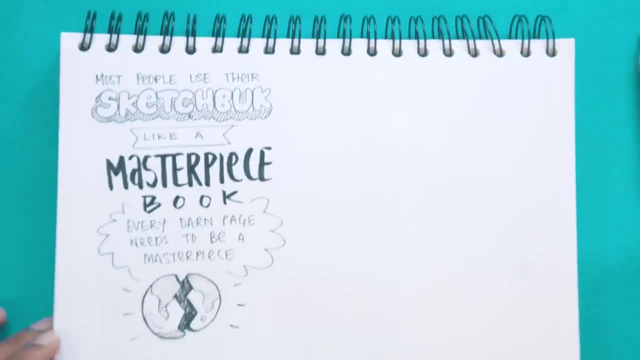 It totally works fine. Number two: make sketchy notes and brainstorms. Most people use their sketchbook like a masterpiece book, like every damn page needs to be a masterpiece or else the world will fall apart. I think it's a debilitating way to. 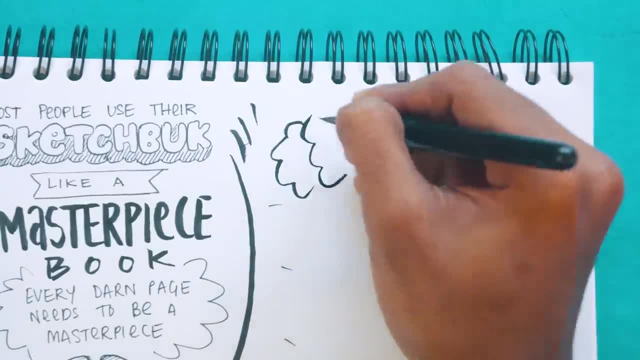 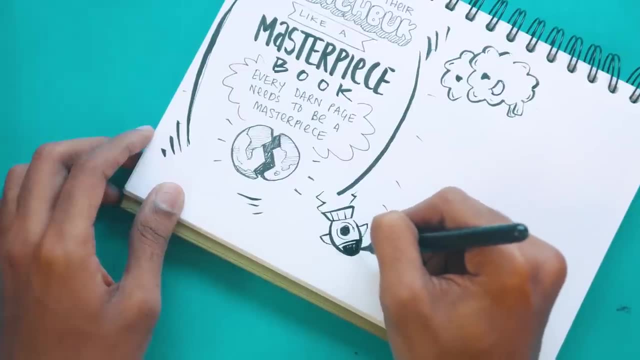 use a sketchbook. to be honest, I use mine to not only make drawings but also to make random notes of ideas and to brainstorm things. And to make these things fun, I try to make my notes a bit sketchy, you know, making visual notes and brainstorms with little doodles here and there. 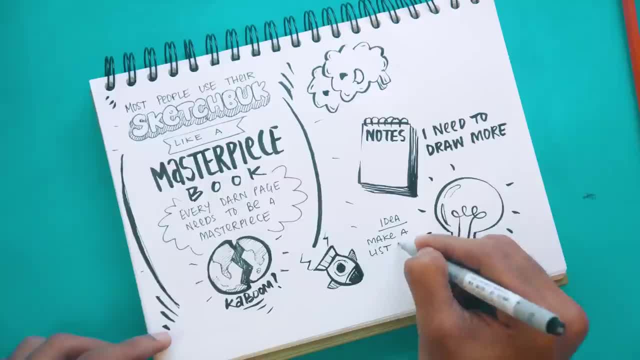 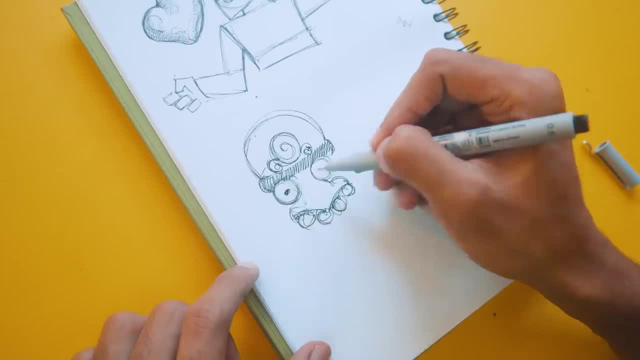 instead of just using words, Because man, oh man picture is worth a thousand words. Number three: do mindless scribbles. Sometimes I just don't draw anything and make random scribbles. Yeah, I just make random scribbles. Yeah, I just make random scribbles. Yeah, I just make random scribbles. 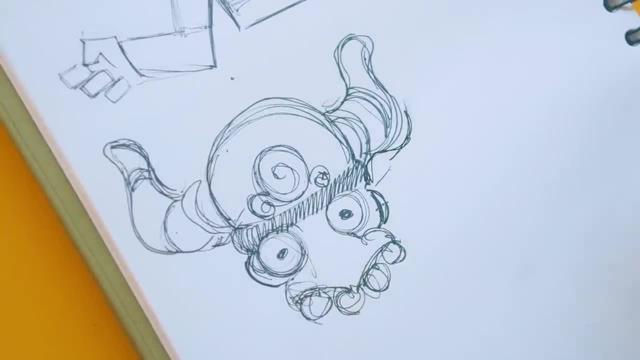 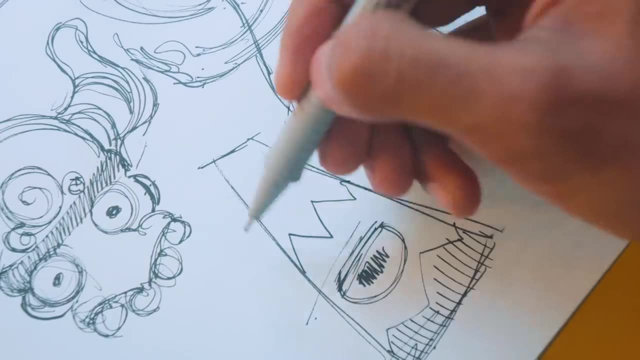 And trust me man, a lot of it is weird, But just filling a page of mindless doodles in a sketchbook is like a good way to fill your page and practice some drawing. And at the same time I gotta say 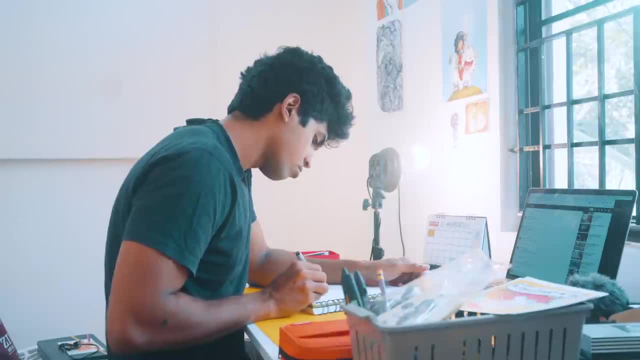 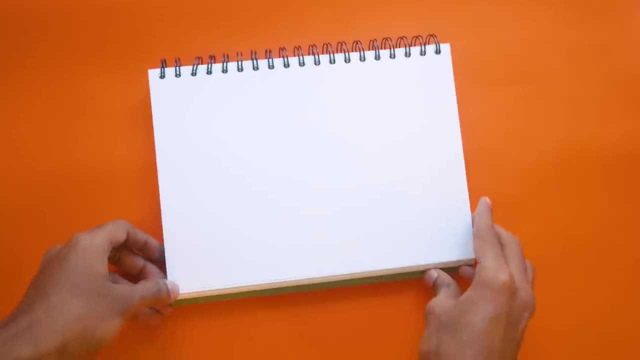 it's very therapeutic, Yeah, like I don't even go for therapy anymore. My therapist hates me, but yeah, I don't go for therapy. Number four: test your ideas. You know, your sketchbook is like a research and development department for your brain. This is actually the. 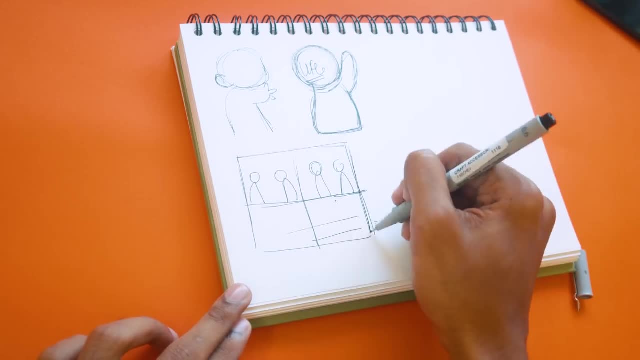 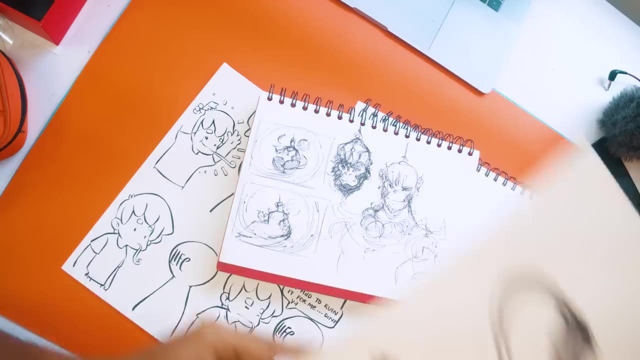 place where you go crazy and test all the things that comes to your head. It's like a lab to experiment new ideas and see if they work. Most of my illustrations first start in my sketchbook. It starts as an idea, where I scribble them out and figure out a way to execute them before me. 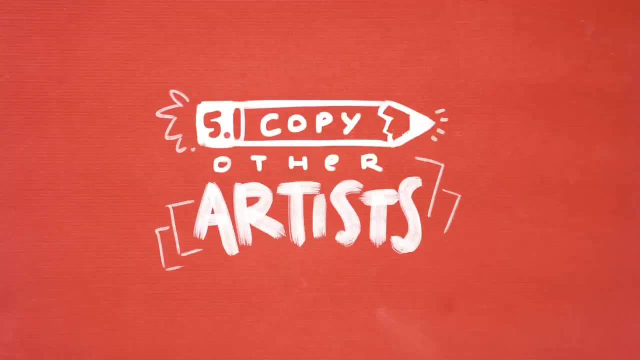 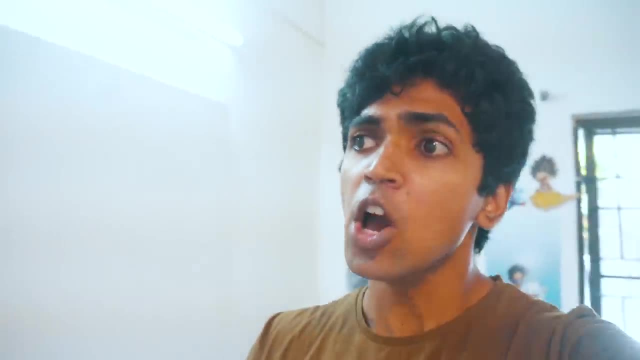 actually going through with it. Number five: copy other artists. Whoa, whoa, whoa, whoa, whoa. wait, just telling me to copy other artists. That is not cool, man. That is not cool. Copying is wrong. 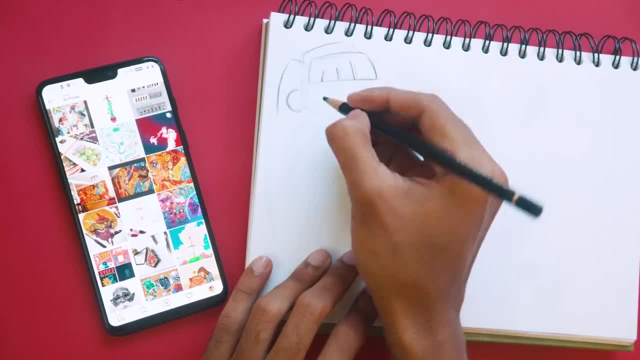 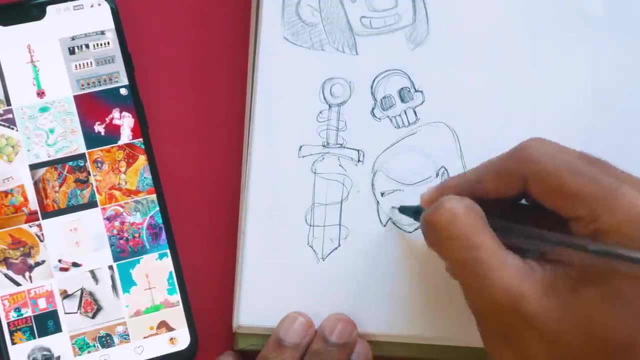 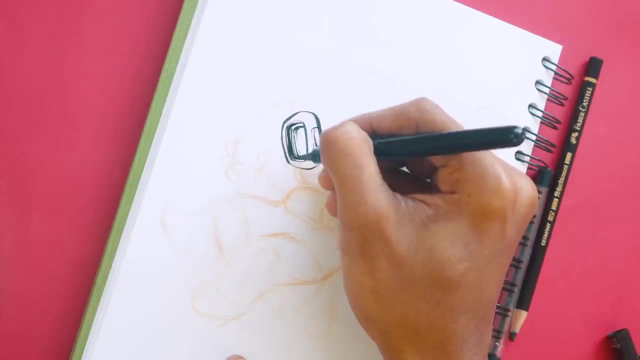 Well, my friend, let me tell you something: If you are copying other artists to pass their work as your own, then no, don't copy. Copying in that case is wrong. But if you are copying to learn from them and to improve your skills as an artist, then it's completely A-OK, Because that is one of 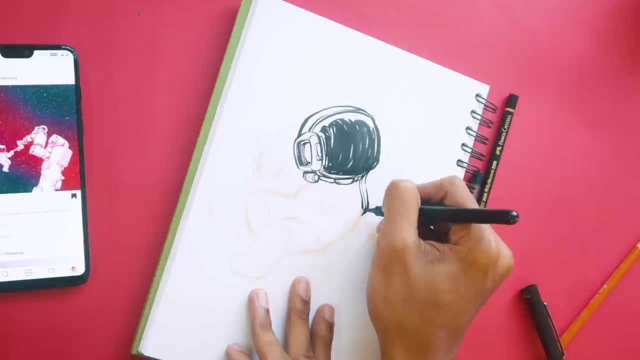 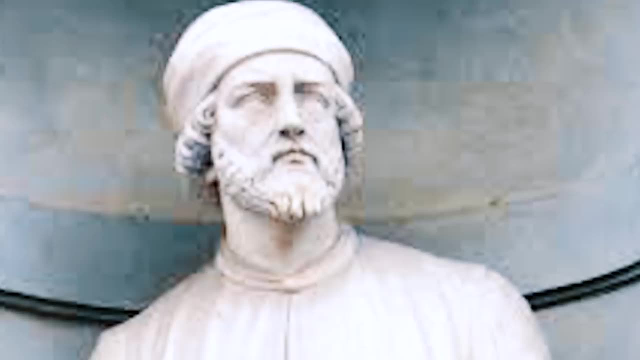 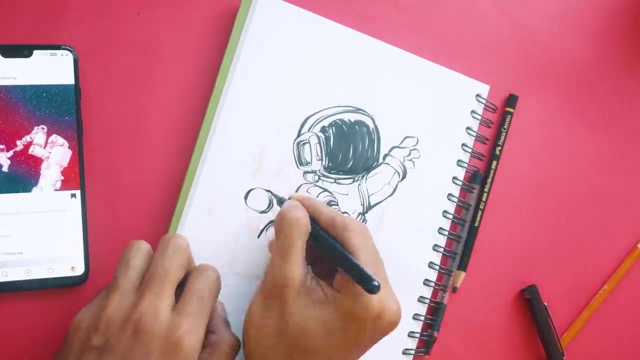 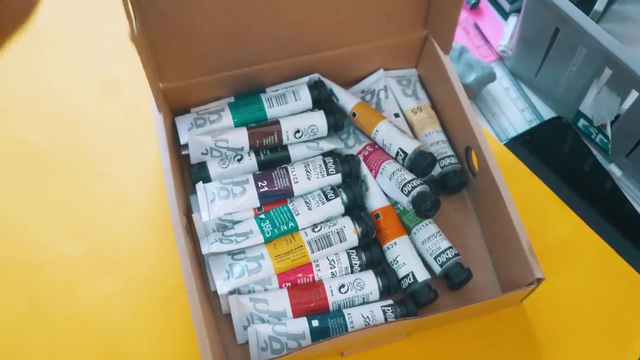 the biggest ways artists learn. It's by copying their masters and mentors and teachers and inspirations. Masters like Leonardo, Donatello, Michelangelo and Raphael all copied from their masters to learn their art. So copy to learn, And that is completely OK. Number six: try new mediums If you are used to. 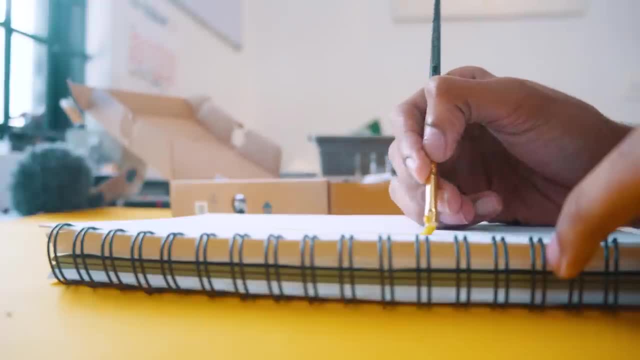 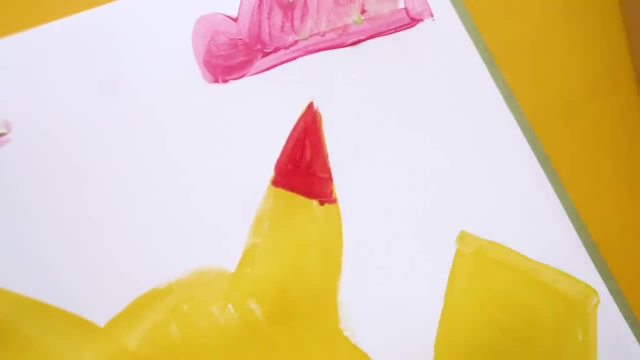 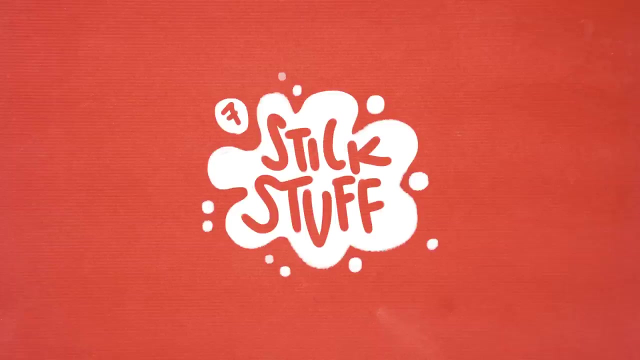 one medium of art, try another one. Test things out and play with it, because you may discover something new and unexpected that will completely change your art and probably even evolve it into something new. Just kidding, Try something new. Try a new medium. Number seven: stick stuff, Yeah. 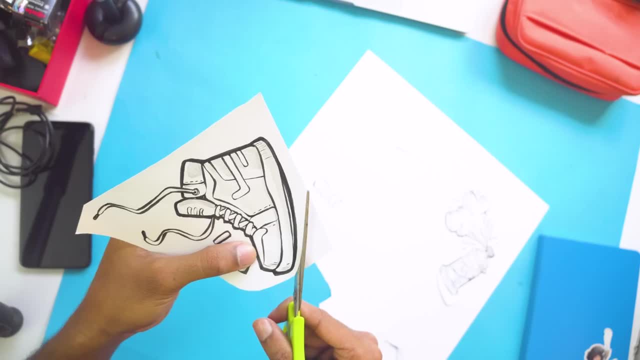 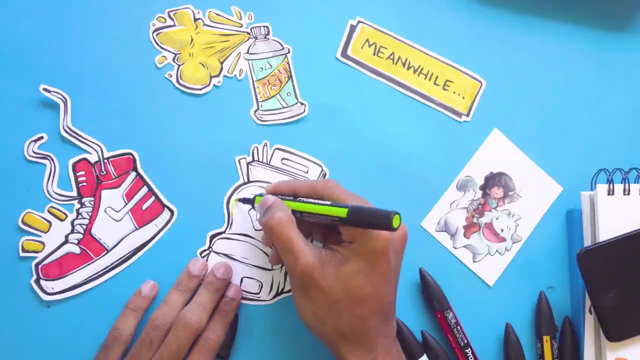 in your sketchbook. This is fairly new to me, but I got to say it's pretty damn fun. You can make your own, cut out pop up stickers and just stick them in your sketchbook and make it look cool. Or you can stick some usual stickers like the rest of the humans do on this planet. 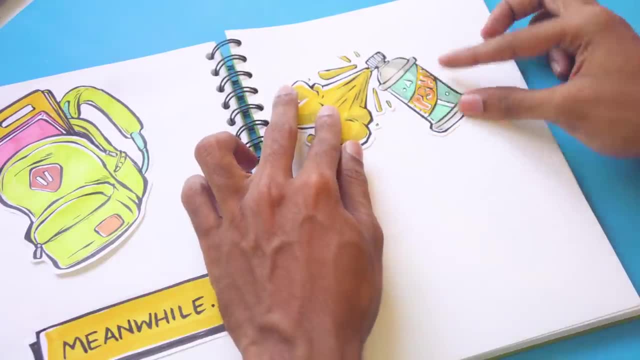 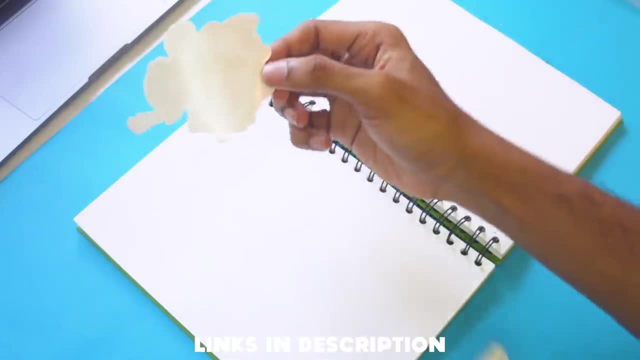 And if you're out of stickers in any case, you can just head to my shop and buy a sticker pack which has totally cool, cool, cool stickers and stick them in your sketchbook, man, Because my stickers are pretty damn cool. Next thing: Enough with the plug. 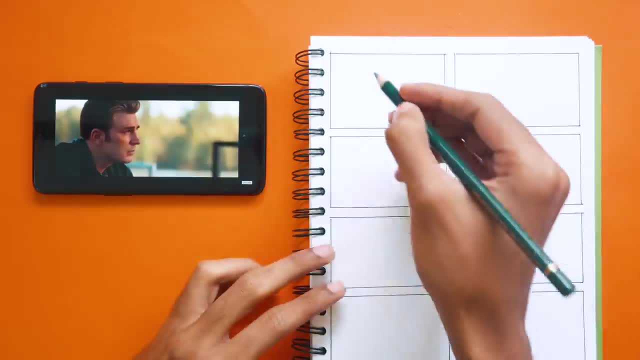 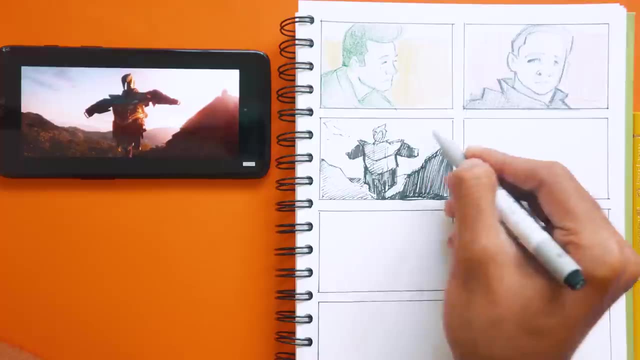 Number eight: draw frames from films. This is something that I've recently discovered: Grabbing stills of some of my favorite shots from a film and drawing them in my sketchbook. As fun and easy as it sounds, it's actually a lot complicated, But if you do this exercise. 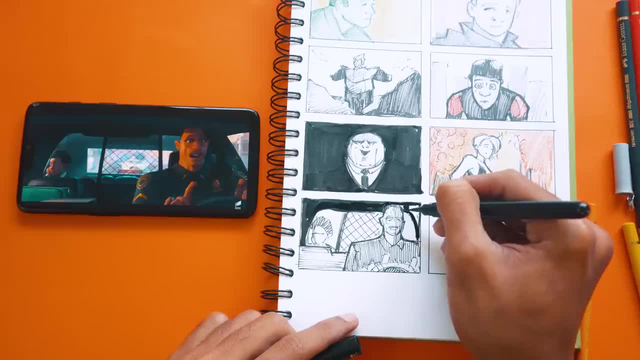 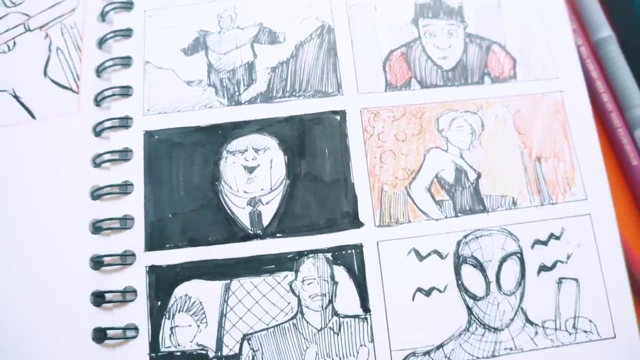 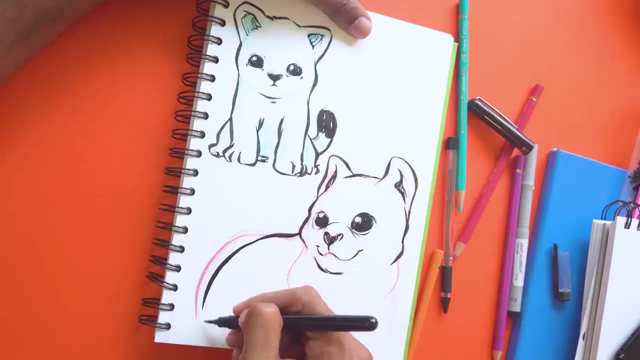 you learn a lot more about colors and compositions, And that, my friend is Tudel Co, And also this makes your sketchbook look really, really nice. Number nine: pick an animal and draw that in your style. Yes, again like it sounds. just pick an animal, pick a random animal.